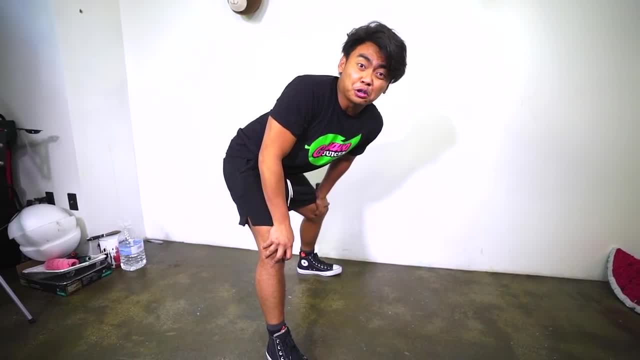 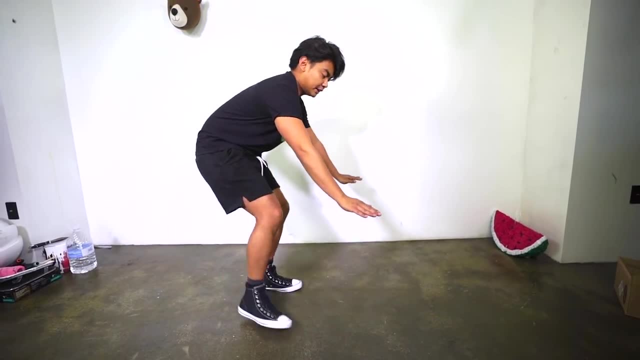 Whoa, Did I do it for real. This whole time I thought it was like really difficult, but it's just all muscle memory. Wow, that is amazing. Here we go, Let's do it again. See Nothing under here. 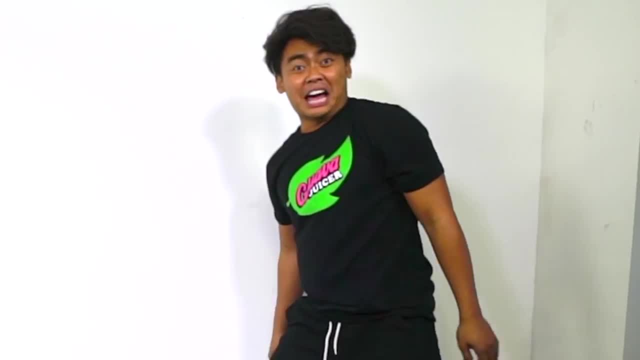 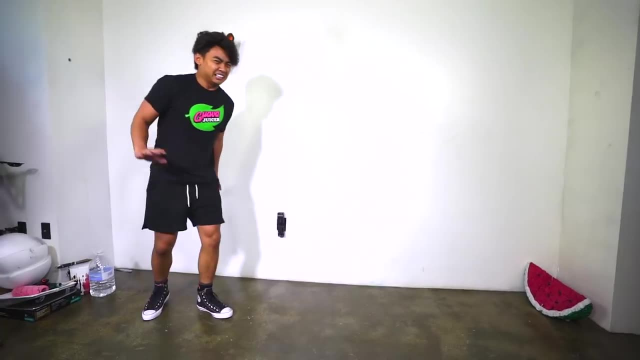 Okay, Okay, here we go. Whoa, Did that look good, or not? Whoa Good, And then just hop A little bit sloppy. but let me fix that. Mm, Mm, Mm, Mm. 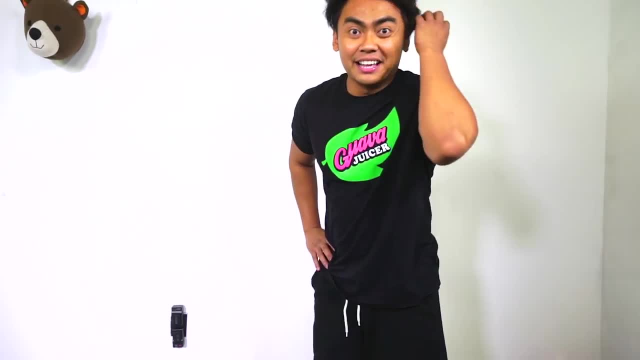 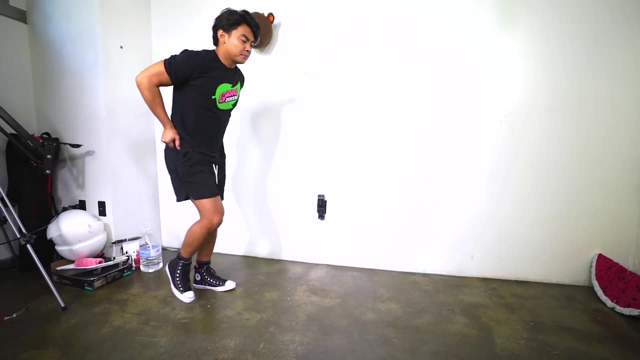 Oh yeah, Mm, It's not perfect, but it's doable. What I'm trying to say is: You can do it too Seriously. Just grab a box, Get that muscle memory And then Ugh. 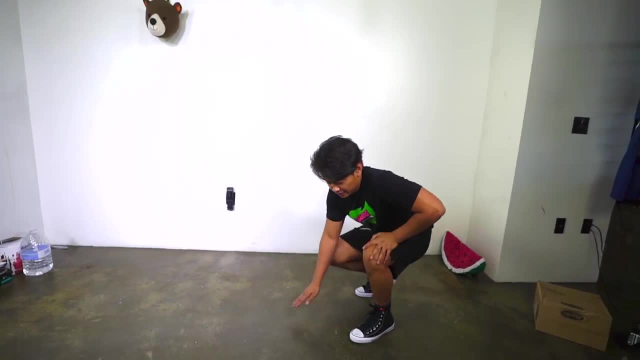 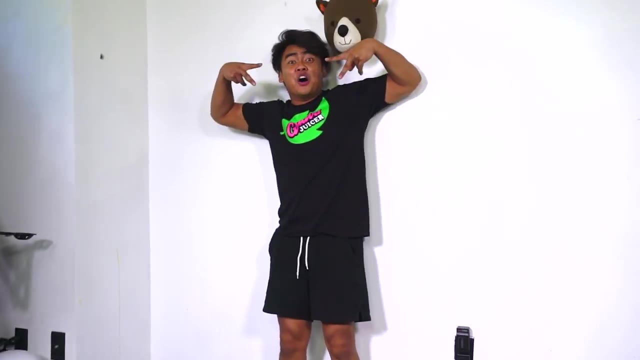 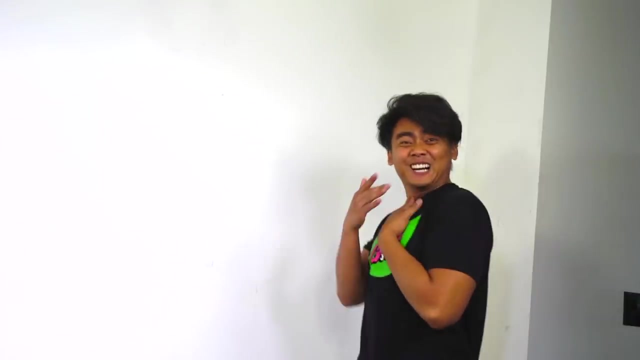 It kind of works. It's very tiring, though, Check this out. This is a, uh, one-centimeter box. Oh Snap, Hey, Half a foot, Nice, Here we go. Oh my God, All right, here we go. 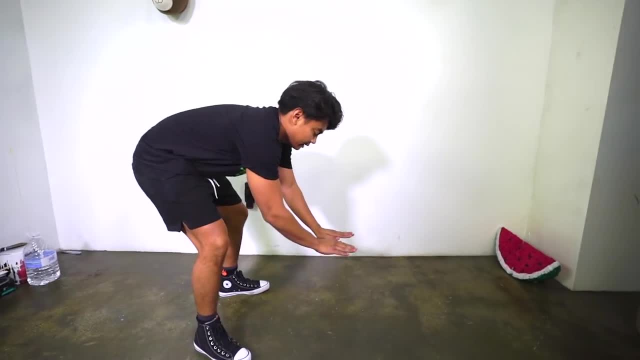 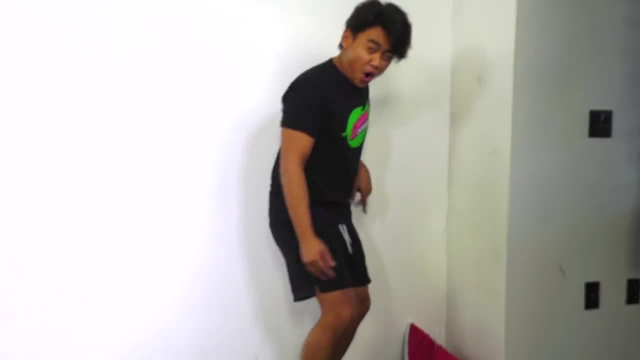 Let's raise the bar a little bit. It's kind of like limbo, but it's not All right raising the bar right here. Here we go. Let's do this thing. Whoa, Oh, I think I'm doing it. 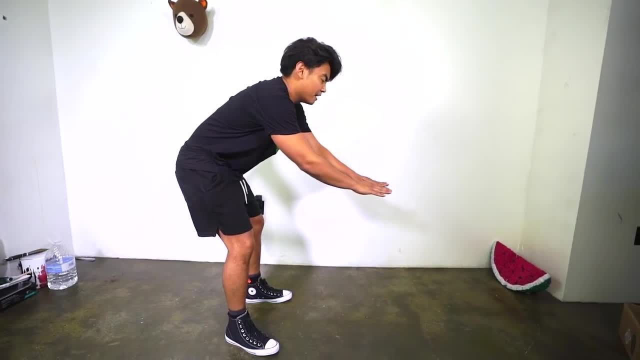 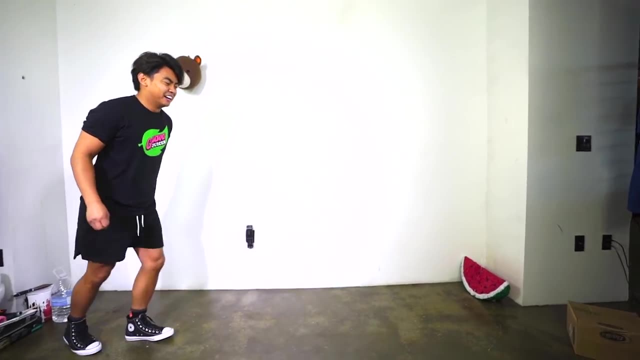 Okay, All right, let's raise it up even higher. Here we go. Might be a little bit too high, but I'll try my best. Here we go. Ow Dang it. I guess that's how you do it, really. 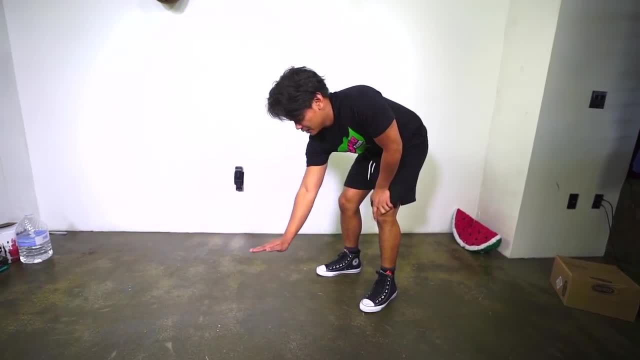 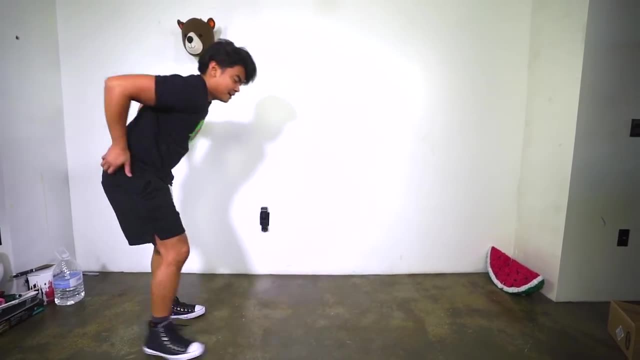 It's easier if you, If you do it lower, because you don't have to jump as high. So do that. Do that again, Nice, Ah, Okay, I think I'm getting tired. It's looking sloppier and sloppier. 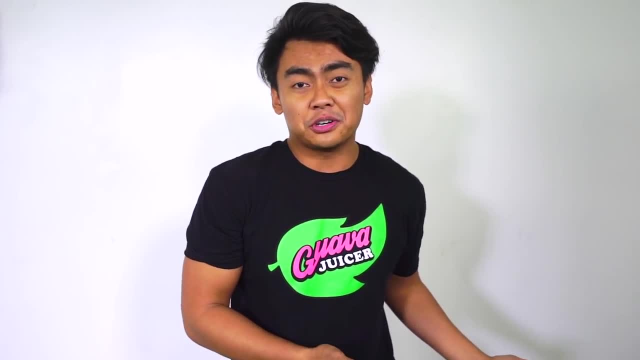 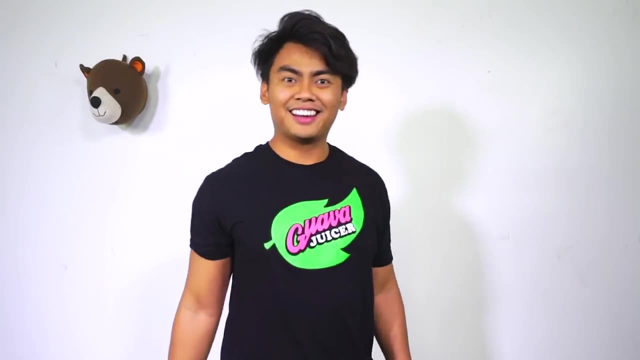 Wow, That's really how you do it. I started this video not knowing how to do it. It's not perfect. Let me do one more for good measures. Here we go, Nice, Nice, Yeah, All right guys. Thank you all for watching today's invisible box challenge. 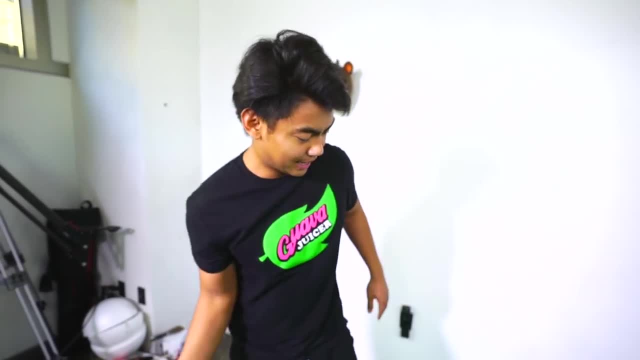 Try it yourself. Let me know if you did it also. Okay, I'll see you guys later. Nice, Perfect Yo. just make sure to, When you edit it, just green screen, the green screen up. Okay, All right. Thank you.